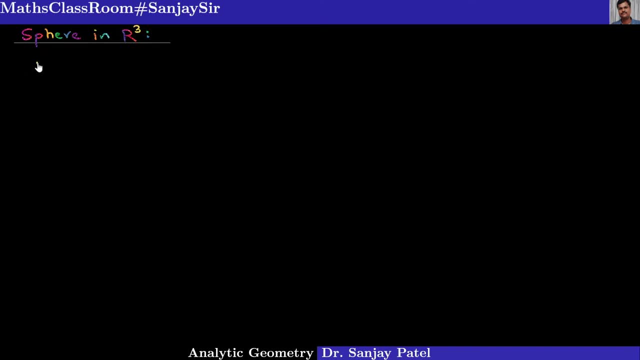 Okay, so let us begin with some examples. one or two examples. Let me take first simple example: Determine whether the equation x square plus y square plus z square plus 2x plus 4y plus 6z minus 11, equal to 0, represents a sphere or not. 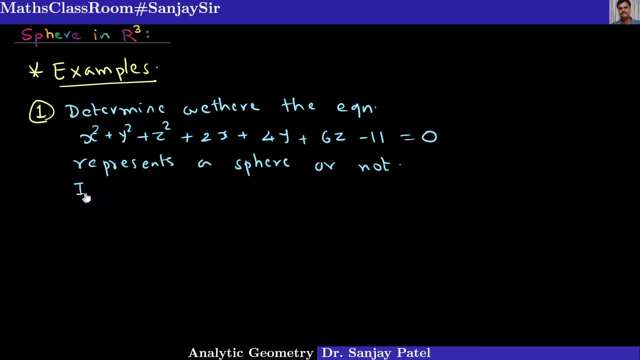 Any fears. Then find its center and radius. Find its center and radius. So let us solve this. First of all, comparing the given equation with the general equation x square plus y square plus z square plus 2ux plus 2vy plus 2wz plus d, equal to 0,. 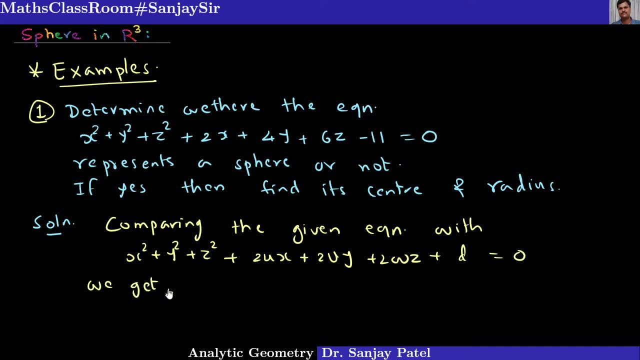 we get 2x. x coefficient is 2 here and here, x coefficient is 2.. So 2v is equal to 2, we get 2u. So when the value of 2 is equal to 1, we get u. 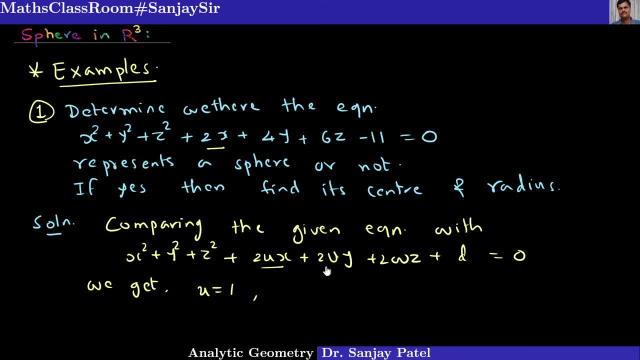 Remember just: whatever is the coefficient given of x, y, z, you have to divide it by 2 to get the values of u, v and w respectively. Like 2v is equal to 4, so v is equal to 2.. 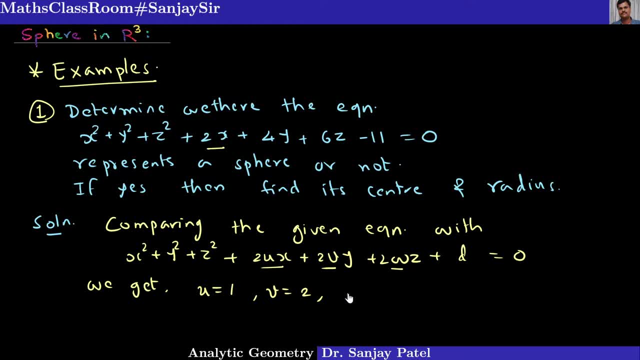 And 2w is equal to 6, so w is equal to 3.. Also, the value of d. This is not the same as the value of 2.. this constant is d. d is equal to minus 11.. So we get these four numbers Now to check. 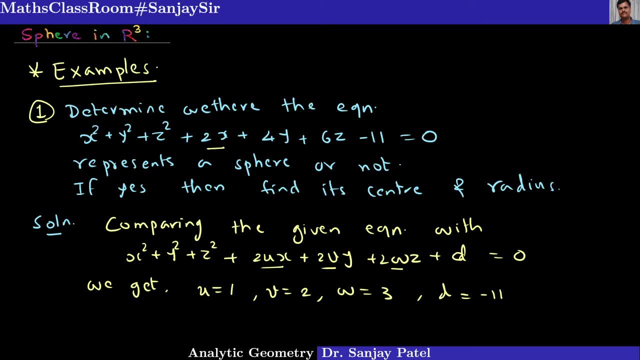 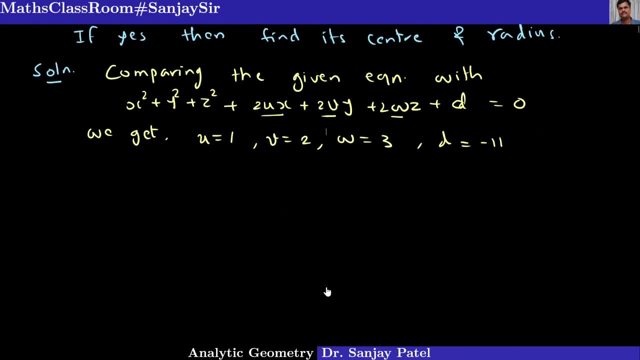 whether it is a sphere or not. we will check that condition. Now you know, the condition is that u square plus v square minus. sorry, u square plus v square plus w square minus d. Let us find the value of this expression, If this expression turns out to be positive. 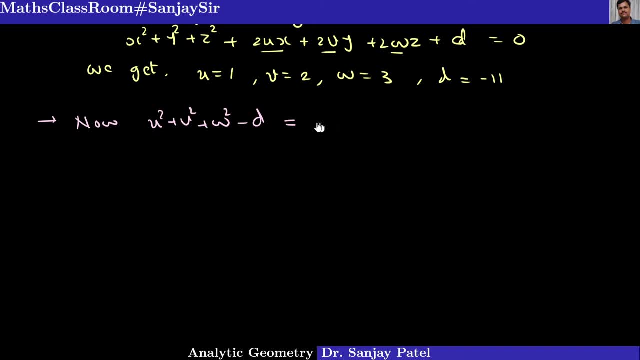 then our given equation is definitely a sphere. So u v, w are 1,, 2 and 3.. So 1 square plus 2 square plus 3 square and minus d, So 1 plus 4, 5.. 5 plus 9, 14.. 14 plus this, minus, minus plus 11.. So this is 25 and it. 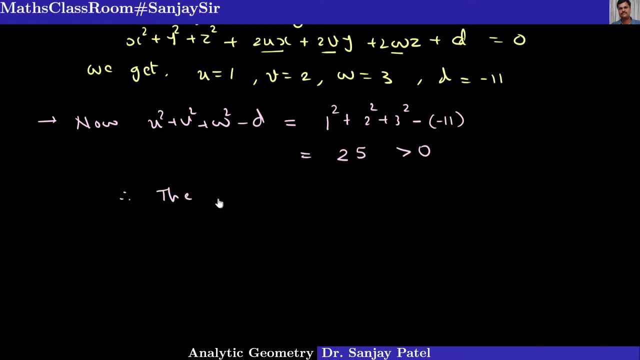 is positive. So therefore, the given equation. given equation is a sphere. Okay, In this case, the center is d. The center of the sphere is c, is equal to minus u, minus v and minus w. What are u? 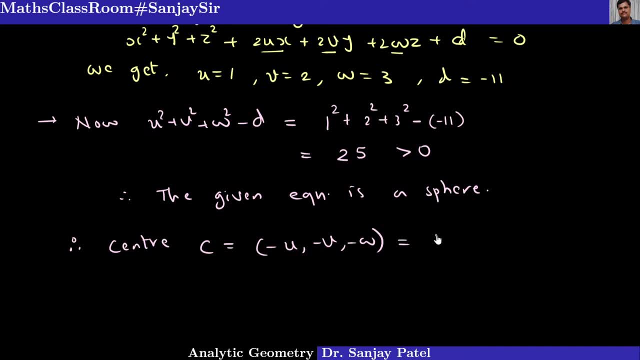 v, w. They are 1,, 2 and 3. So the coordinates of the center will be minus 1,, minus 2 and minus 3.. So from the given equation also you can directly find the center. That will. 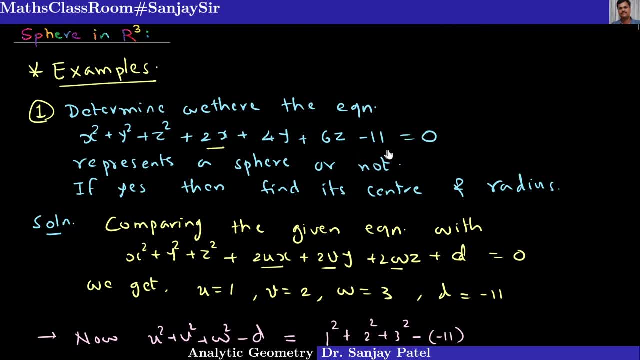 be very useful in future. So suppose this type of equation is given and you are told that it is a sphere, And find the center and the radius, Just divide the coefficient of x, y, z by 2 and change its sign. If it is plus, make it minus, If it is minus, make it plus. So here it is. 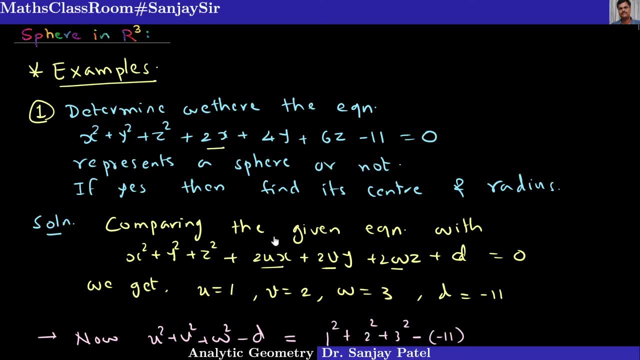 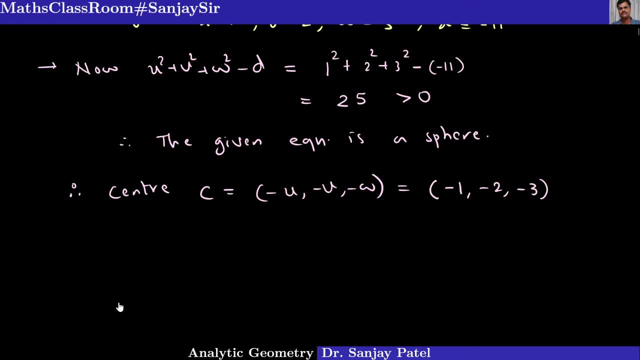 minus 1, minus 2 and minus 3.. That will be the center And finding the radius, just take the positive square root of this condition. So the radius will be. I can write like this: radius a is square root of u square plus v, square plus w square minus d. So it is. 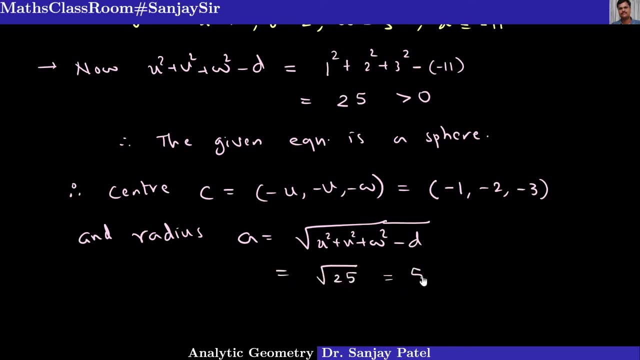 nothing but square root of 25 and it is equal to 5.. So radius of the sphere is 5.. So the problem is solved. Let us take another example based on the basic theorem Or the basic general form of sphere. So second example, example two: Find the Cartesian. 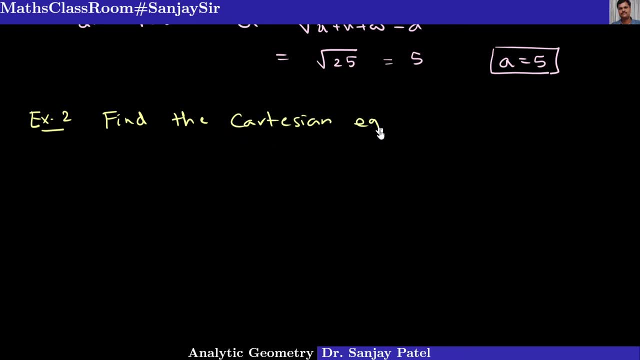 equation, find the Cartesian equation of a sphere, of a sphere which is passing through, which is passing through A, the point B, then the point C and the origin 0,0,0.. Remember, to derive the equation of a sphere, you should have center and radius. 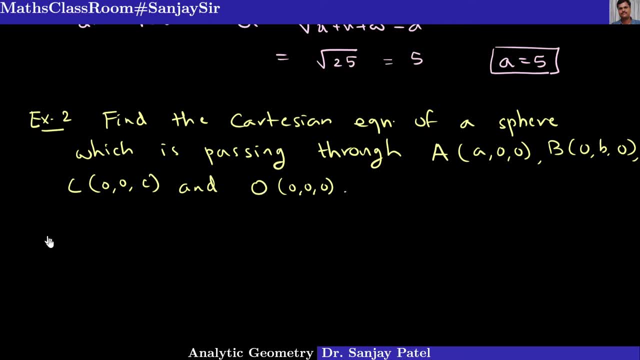 The center and radius are not given in this example. And also remember that whatever equation we are going to derive in this problem, that is very useful. So you can remember this final equation of the sphere for the future purpose. Okay, Now to derive the equation in this example. we assume that suppose the required sphere is given by: 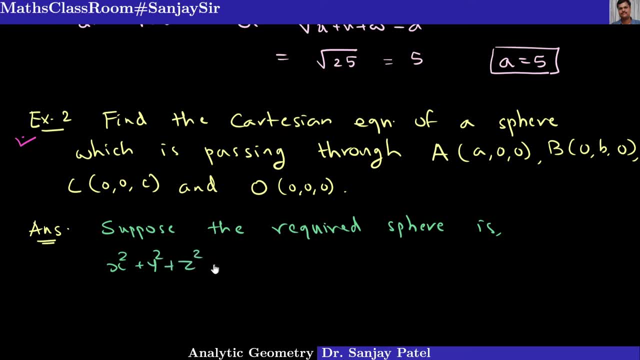 x square plus y square plus z square plus 2 ux plus 2 vy plus 2 wz Plus d, equal to 0.. Okay, And let us call this sphere as S. S, then colon means: this is the label for this equation, or the name of this sphere: S. 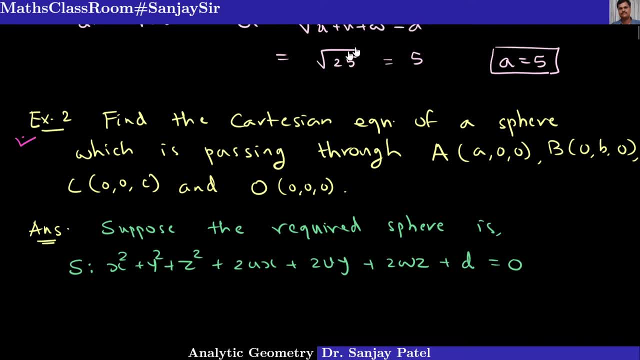 Okay, Now we know that this 0,0,0.. As the point 0,0,0 lies on the sphere, So I can write like this: This is our understanding. 0,0,0 belongs to S. 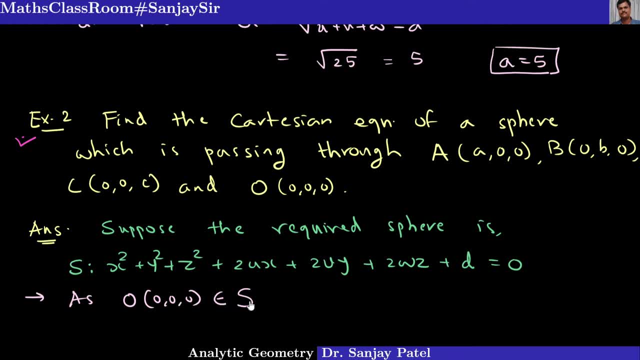 0,0,0 belongs to S implies this point must satisfy this equation of the sphere We must have. you can put x equal to 0,, y equal to 0. So you will get 0 square That is 0,0,0, because x, y, z are 0.. 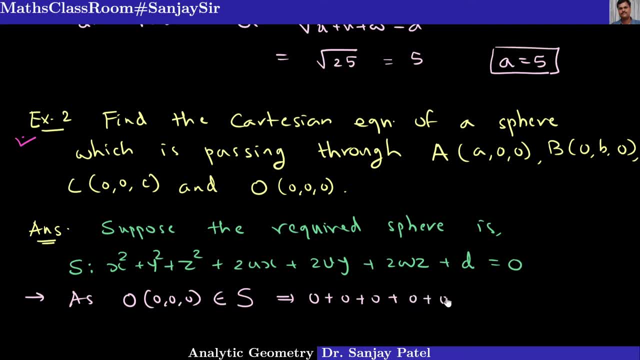 These three terms will also be 0.. We will also be 0 because it is containing x, y, z plus d equal to 0. So, as a result, we are getting d equal to 0.. Remember, we assume that the required equation of the sphere is this, and we don't know what. 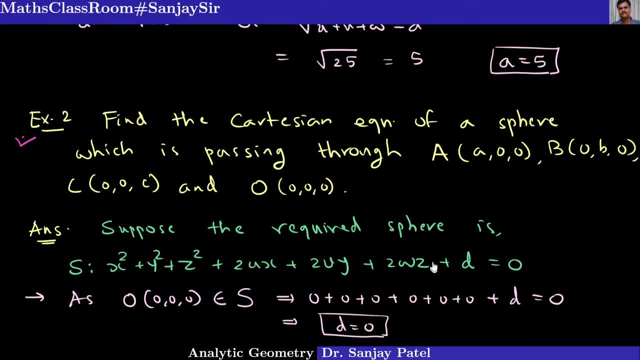 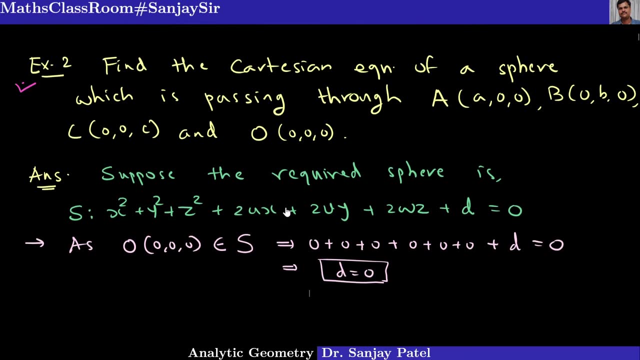 are these constants c, v, w and d. So our job is to find these numbers, and we have got the first number d in this, using the condition that this, This sphere, is passing through the origin. Now this sphere is also passing through the three numbers a, b and c. 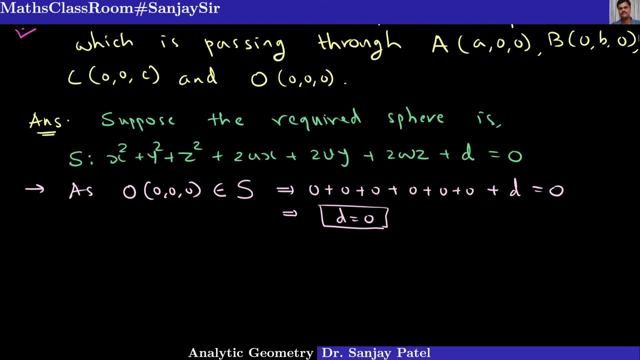 I will be using another condition. Also, the point a, a 0, 0 belongs to the sphere S. Okay, So this implies I can put x equal to a, y equal to 0 and z equal to 0. So we will get a square plus 0 plus 0 from this equation. 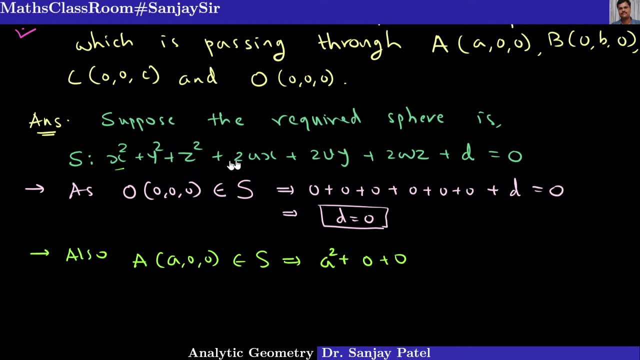 x equal to a, y is equal to 0, z equal to 0.. And here plus 2ua, okay, plus 0, plus 0 and d, We already obtained the value of d, so I can substitute that plus 0 is equal to 0. 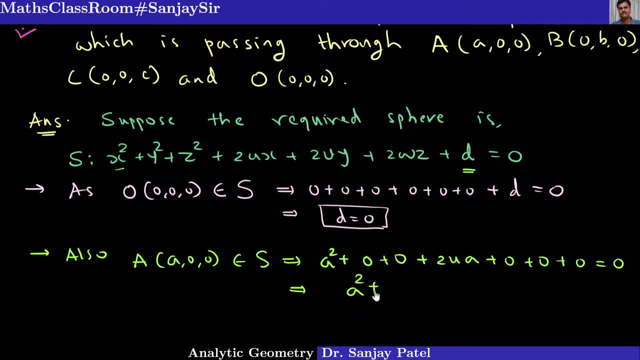 So what I will get from this is a square plus 2a- Okay, Plus 2ua- equal to 0.. So that gives me, that gives me the value of u. So I will get: u is equal to minus a by 2.. 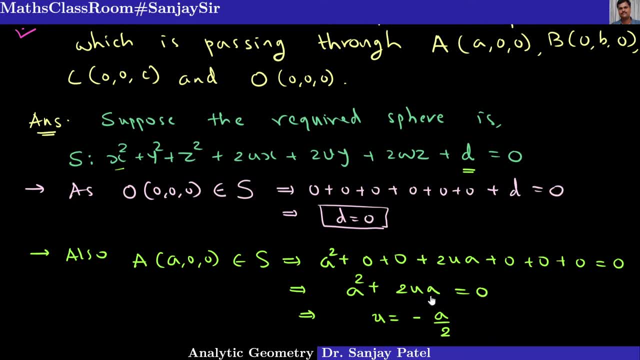 Taking this a square on this side and cancelling 1a, So we will get: 2ua is equal to, rather, 2u is equal to minus a, So u is equal to minus a by 2.. This is my value of the constant u. 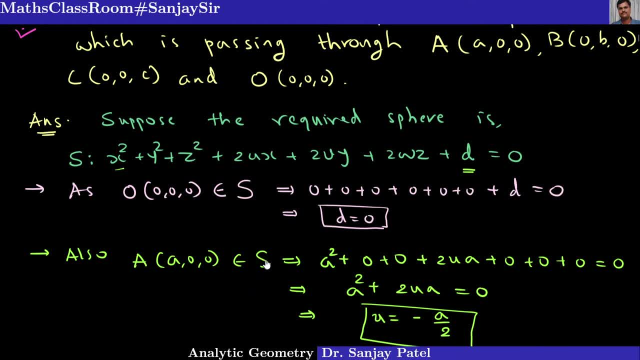 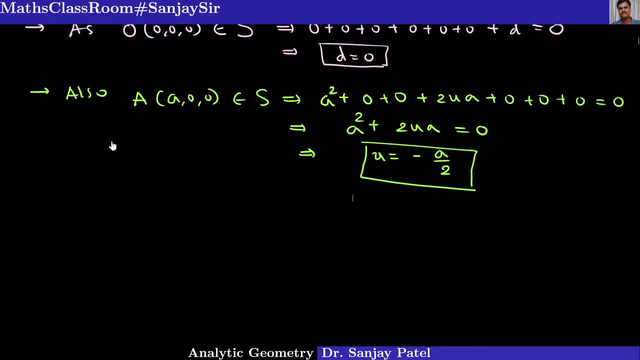 The same way I can find the values of v and w by putting b and c. This remain in two points in the equation of the sphere. So I am not going to write every step, Just you can verify. So I am writing similarly. 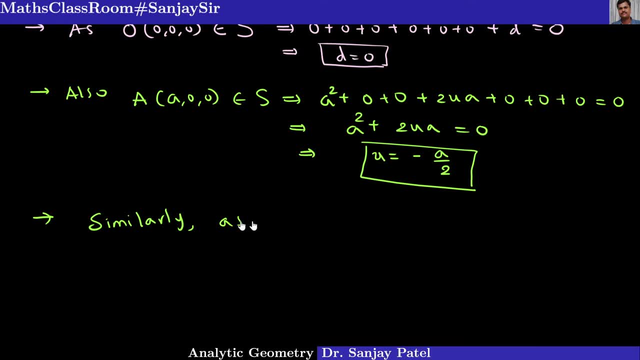 Similarly, As b and c also belongs to the sphere s We can get, We can get. the value of v is equal to minus b by 2.. And value of w is equal to Sorry, And w Is equal to minus b by 2.. 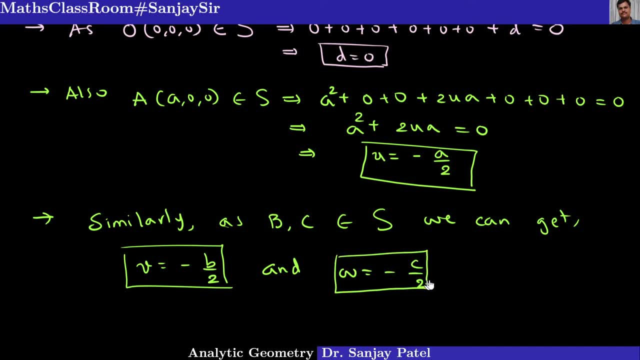 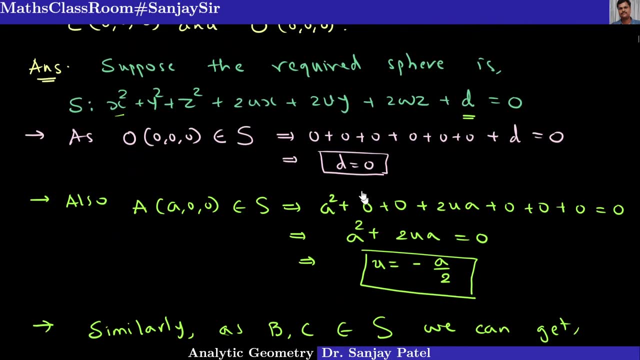 So we have obtained all the required constants in that equation of sphere which we wanted to find. So in this equation now we are substituting the values of u, v, w and also d. d is equal to 0.. u is equal to minus a by 2.. 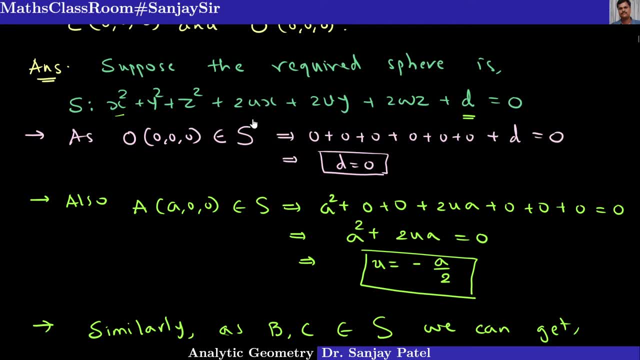 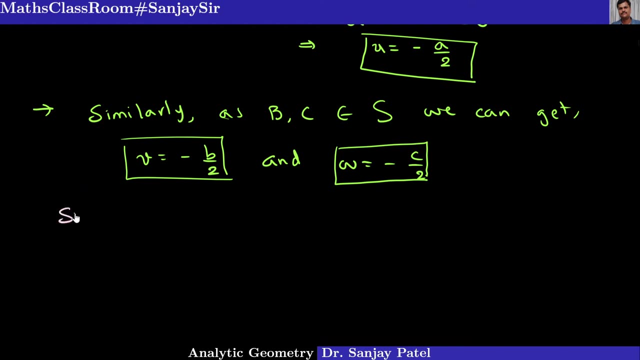 So this 2, 2 gets cancelled. So let me call this equation as star, So putting the values of u, v, w in star. So Substitute The values Of u, v, w and d In star. 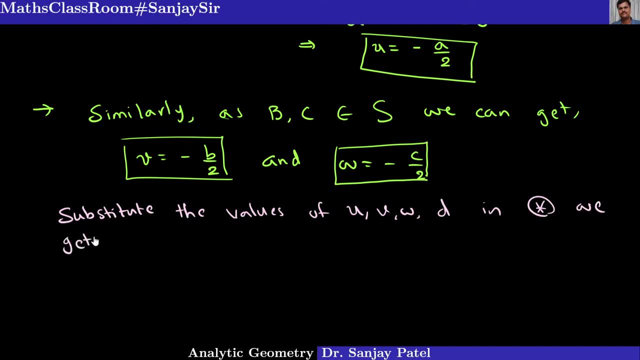 We get. We get x square Plus y square Plus z square. Then minus 2 u x u is equal to minus a by 2. So we will get Minus a x, Similarly minus b y, Minus c z. 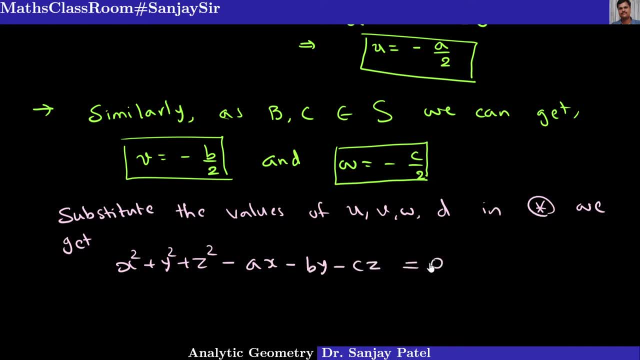 And d is equal to 0.. So we will get: only is equal to 0.. So this is very important equation Of a sphere Passing through 4 points: a- a- 0- 0.. b- 0, b- 0.. c- 0- 0- c. 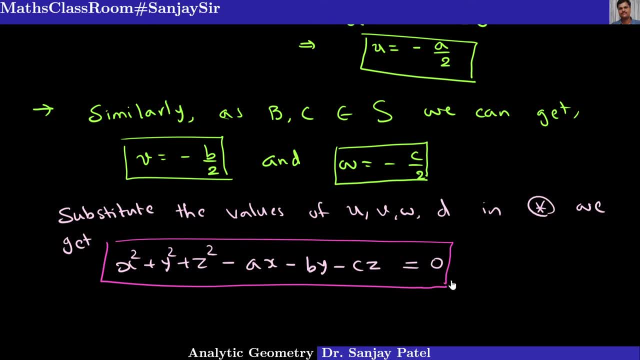 And The origin: 0 0 0.. Ok, Now we will be discussing Intersection of Sphere And A plane. Ok, So Before we discuss The intersection of sphere And a plane, Let us recall: 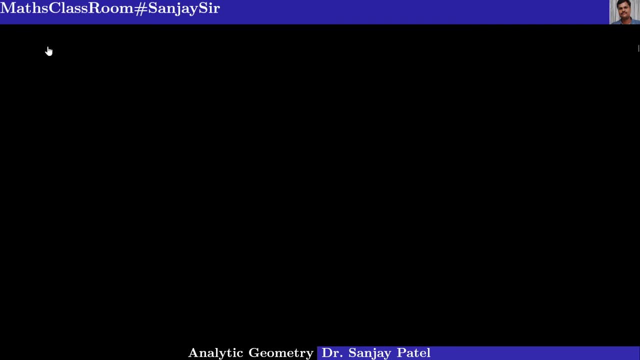 Let us recall the Formula To find The distance, Perpendicular distance Of a point Outside Of a plane. So Let me say Intersection Of A sphere And A plane. Intersection Of a sphere. 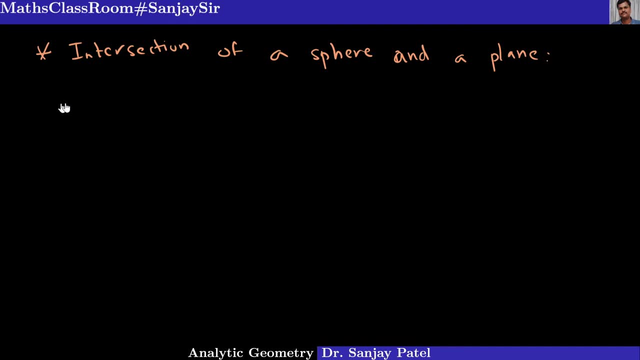 And A plane Ok. So First of all, Note that If we have, Say, a plane, Let me Consider Plane Ok. And A point: Here is A plane Outside Of this plane, Say: 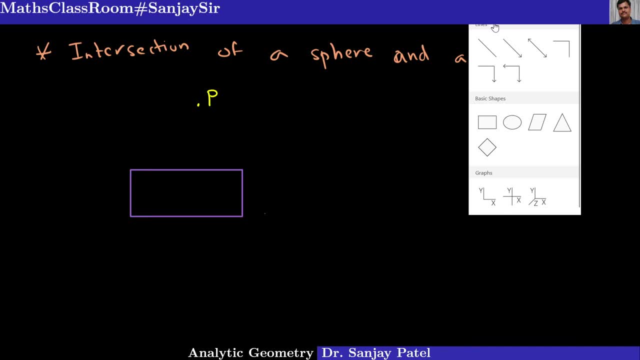 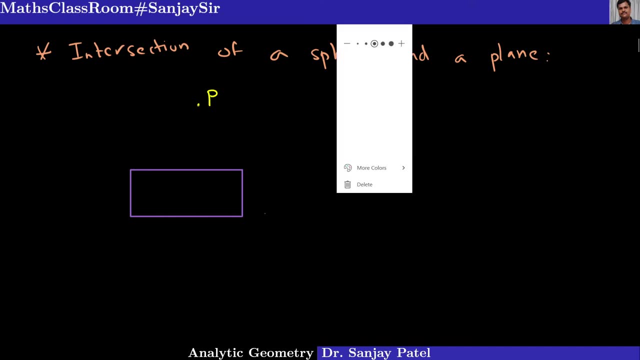 P, And If we draw Perpendicular From this Point Onto This Line? Just a minute, Ok, Let me. Yes, So Draw Perpendicular From this Point Onto This. 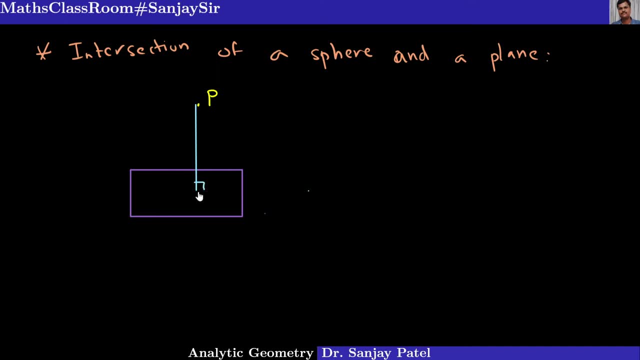 Plane And Suppose The foot Of the Perpendicular Is M And We want To Know What Is The Formula To Find The Plane Is, Say A, X. 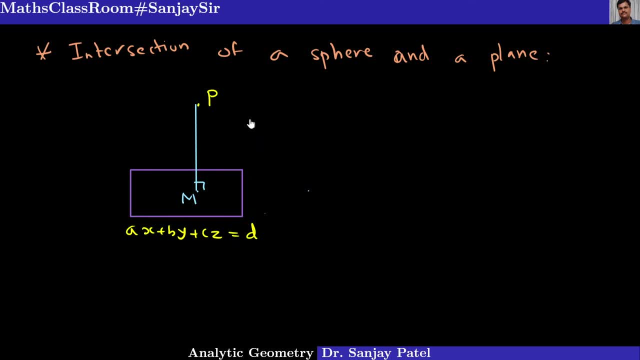 Plus B, Y Plus C, Z Is Equal To D And The Coordinates Of The Point P, Which Is Outside Of This Plane, Is Of A. 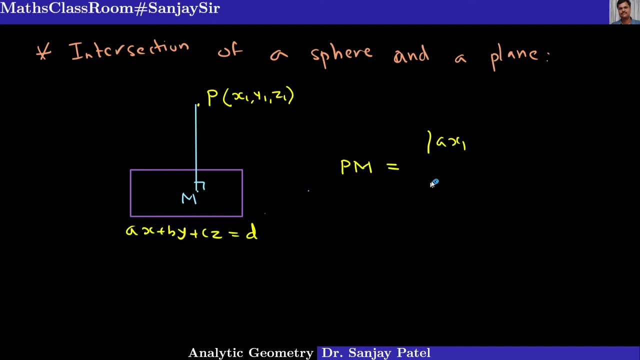 Into X1. Just Subtitute X1. Y1. Z1. In This Equation And Write Like This: A Into X1. Plus. B Into Y1. Plus. 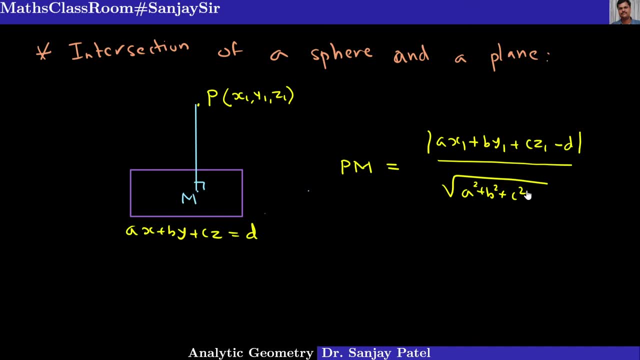 C Into Z1. And Take The Distance Of A Point From Plane. OK, So Using This, We Will Be Discussing The Intersection Of Sphere And. 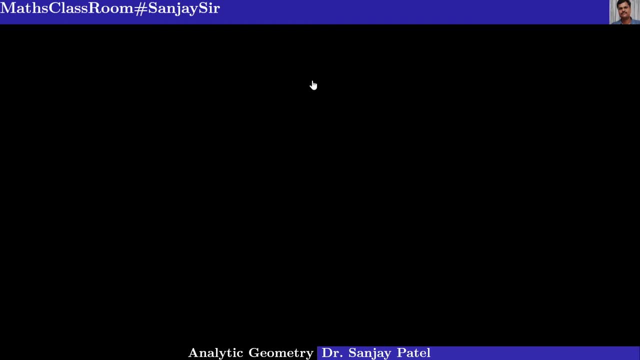 Plane. What Do You Think If Have A Sphere And Consider a sphere in R3 as the, as this equation, x square plus y square plus z square plus 2x plus 2vy plus 2wz plus d, equal to 0.. Remember that throughout the chapter. 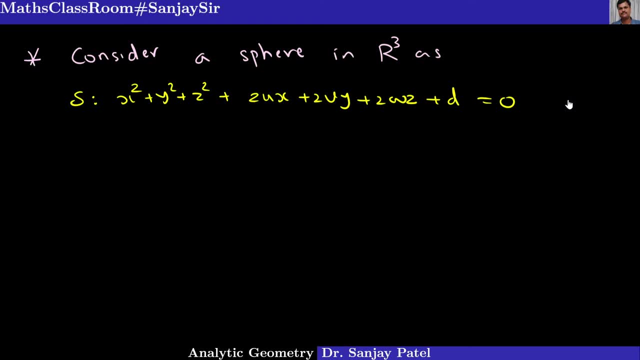 the general equation for sphere in the Cartesian form, we are going to consider like this and will be label as S, If you have more spheres enable, as S1, S2 and so on. So i'm taking a sphere and and I am taking a plane and plane in R3, and this plane will be denoting by always a symbol. 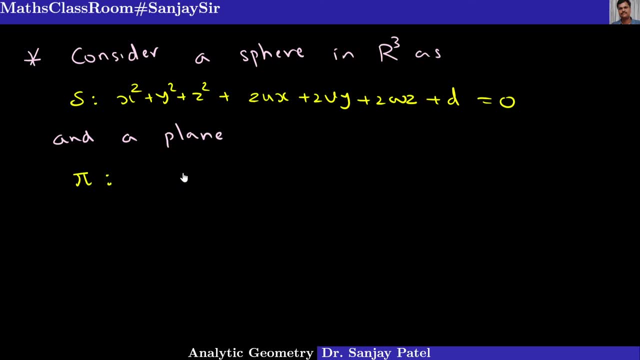 pi pi stands for the label for plane, and this equation of the plane I am taking as Ax plus By plus Cz and is equal to- I will be writing now k, because d is already used here. So we have these two equations. This equation number one is the equation of sphere and equation number two is the equation 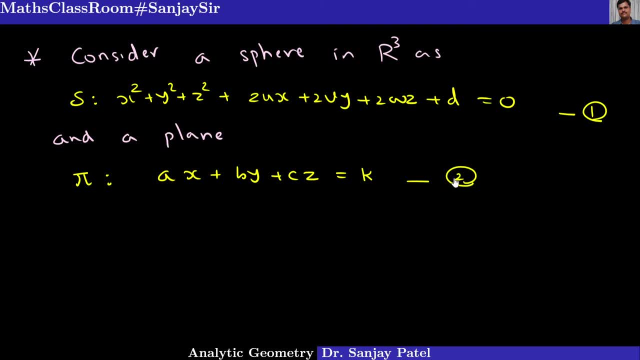 of plane. Remember, both are set of points, So we want to discuss the intersection of these two sets. Okay, Remember the center of this sphere. Just note that the center of the sphere, the center is given by C, whose coordinates are minus U, minus V and minus W, and the radius: radius, if I denote it by R and the radius. 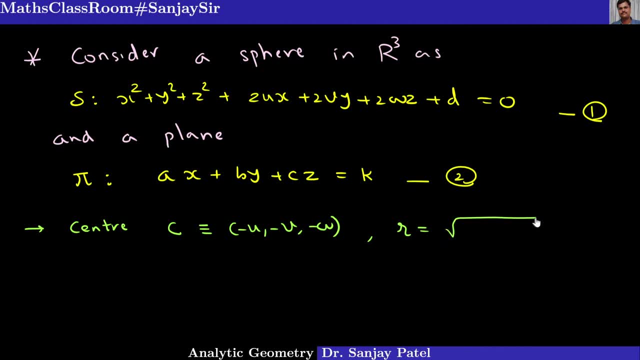 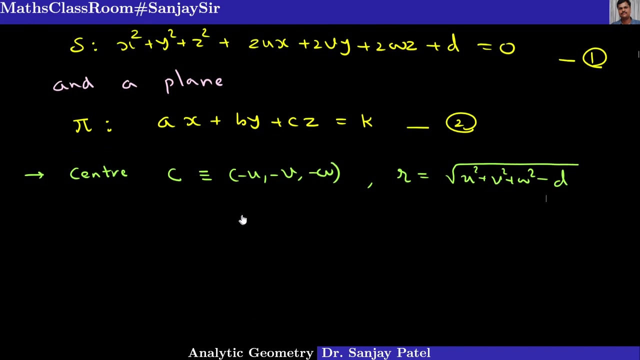 of the sphere, which is given by question number one. you know the formula now: it is U square plus V square, Okay, Okay, Okay, Okay. U square plus W square minus D. Okay, Now to understand the intersection of sphere, and the plane will be dropping a perpendicular. 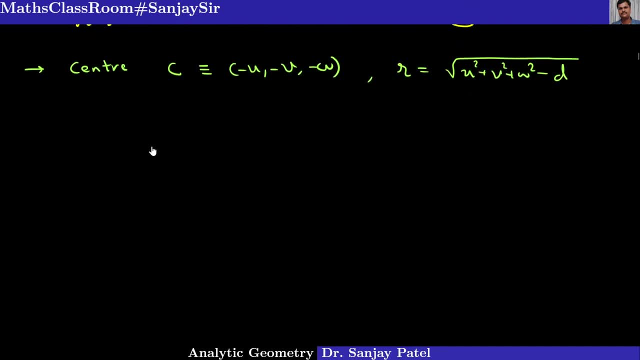 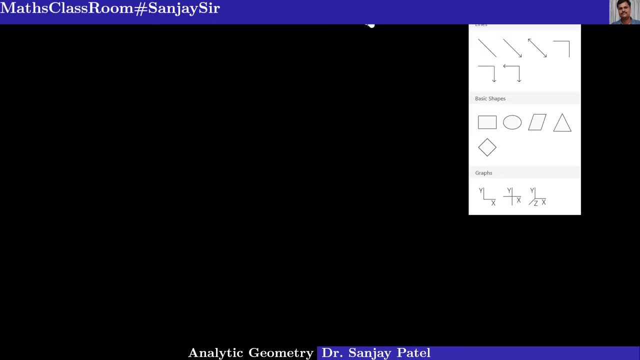 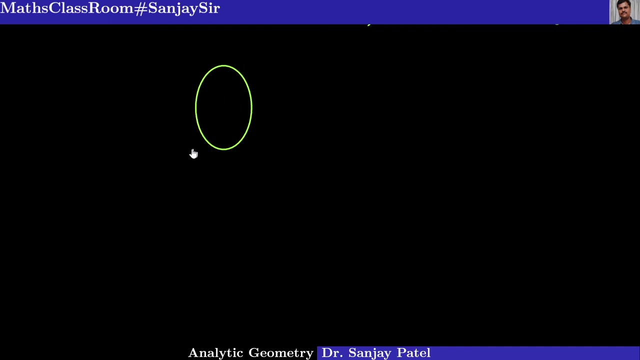 from the center onto the plane. So let me explain by the figure. Okay, I am taking a sphere, So suppose a sphere is given and a plane is also given. So I consider a plane. Okay, And let me extend this, This is a plane. 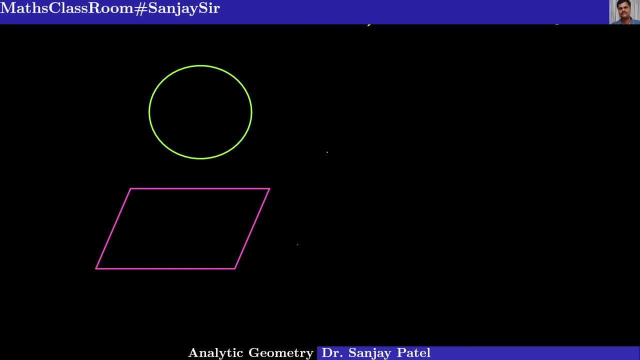 Now we draw perpendicular from this center of the sphere, which is C, onto this plane. Our sphere is S and the plane is pi, So let me show that this is actually a three dimensional object. by drawing a circle like this, Now we draw a perpendicular from the center onto the sphere. 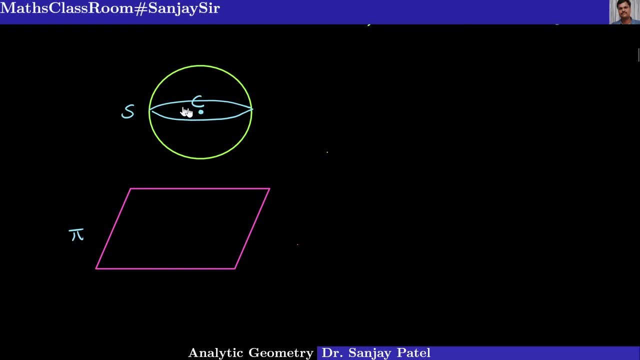 So like this: Okay, This is a perpendicular of. let me Okay, Okay, Okay, let me remove this. yes, let me change this point and suppose this is the center and the foot of the perpendicular is m. ok, this is the center. 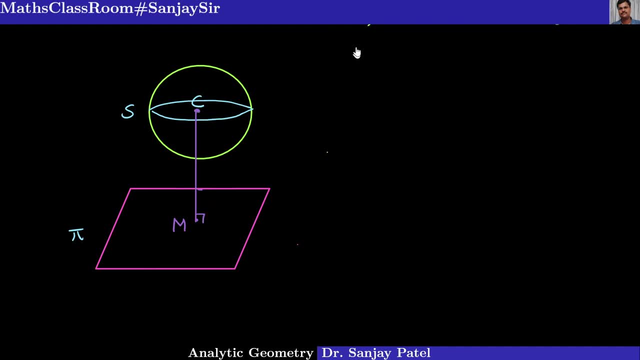 and this is the perpendicular. you know that this thing is the radius of the sphere. this is the radius of the sphere. cm is the perpendicular distance. so this is also this much is also the radius. and this distance, cm, is bigger than the radius. so obviously, in this case, 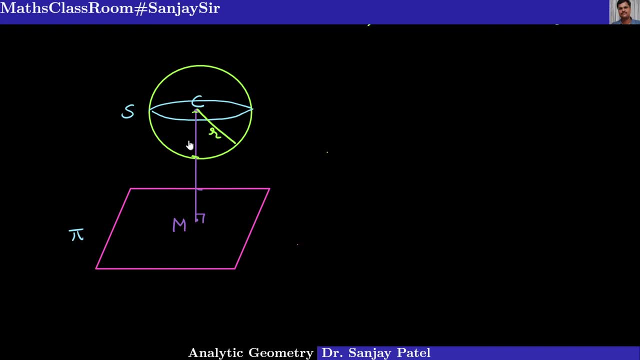 if this situation arises, you can say immediately that the plane is not intersecting the sphere. we can have different situation. this is the one case. you can note down that in this case, in this case, the cm distance, cm is greater than r, so the intersection of plane and. 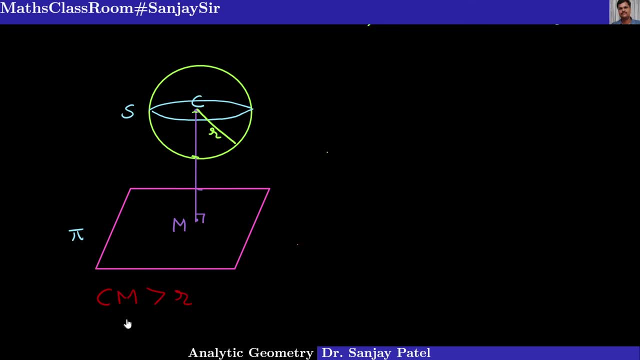 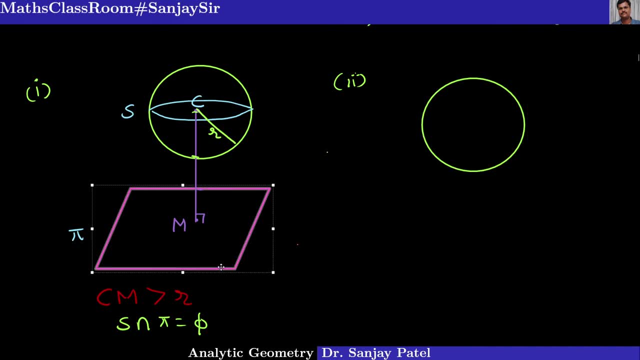 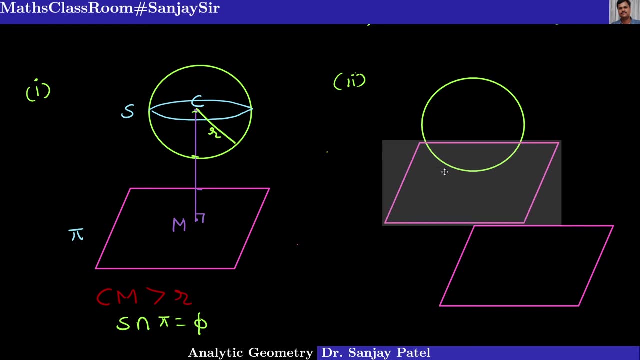 this is. i am also copying this, i am also copying this and keeping over here. now, in this case, this is my sphere, with center c and radius r. ok, and i have a plane like this, say like this: this is a plane, so ok, push it, let me. 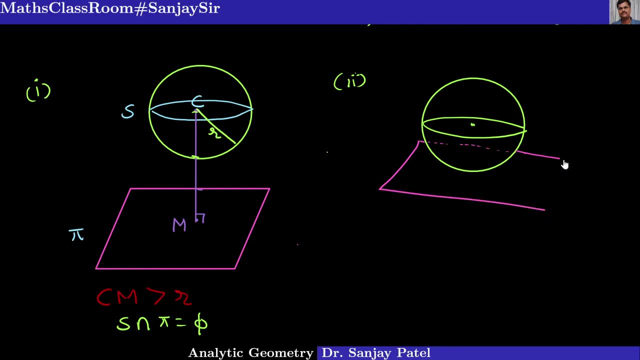 draw this. yes, ok, so this is my plane and we draw perpendicular from the center, and so that this is my plane, we will get this perpendicular distance, cm, which is same as the radius of the sphere. so in this case we have cm is equal to r, so 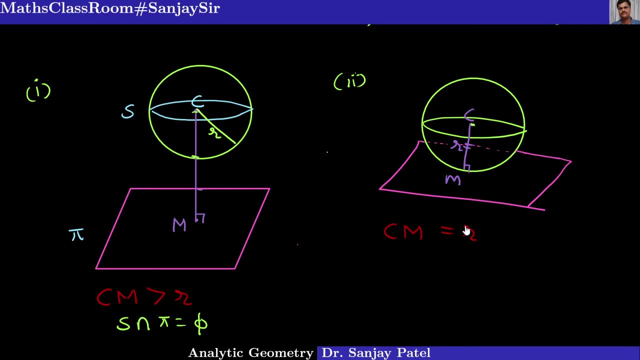 the plane is just touching the sphere, so intersection is only this one point, which is m, or you can say p, whatever so in this case i can write s intersection: pi is equal to say m, not p. it is equal to m, so i can say the plane. 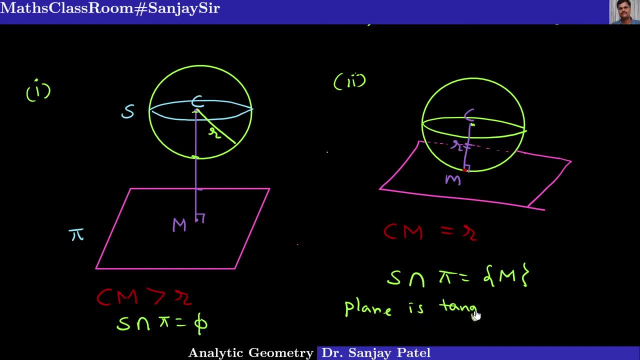 is tangent or is touching is tangent to the sphere in this case. so what you have to do is to discuss the intersection of sphere and plane. first of all, find out the center and find the perpendicular distance of the center from the plane by that perpendicular distance formula which we had. 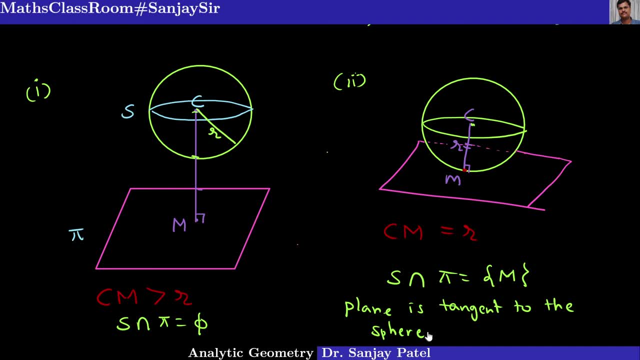 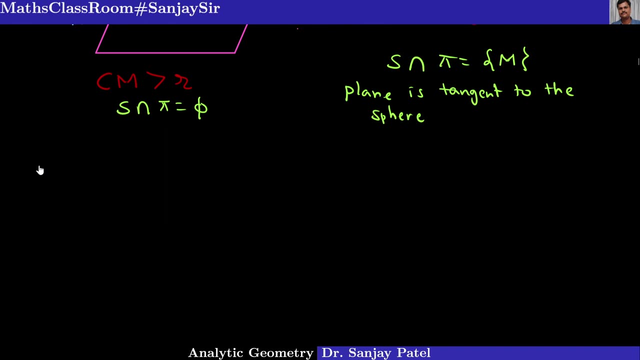 discussed earlier, and then check whether the perpendicular distance cm is greater than r or is equal to r or less than r. what will happen if the distance is less than r? so that will be our third case, and an important case. so the third case is that we have 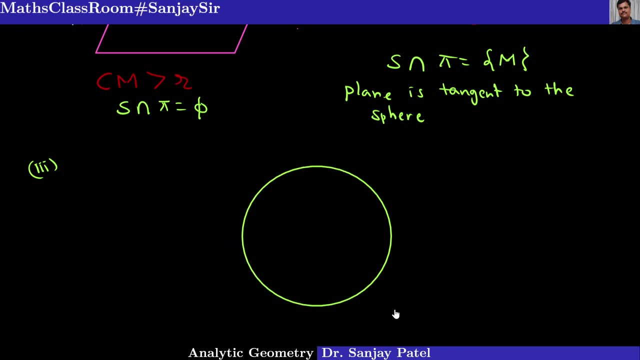 a sphere like this, with center c- and let me draw this, this is a sphere s- and we take a plane like this, say ok, and this plane, you know it is cutting the sphere in many, many points. so there are three situations, as you can immediately understand, which is 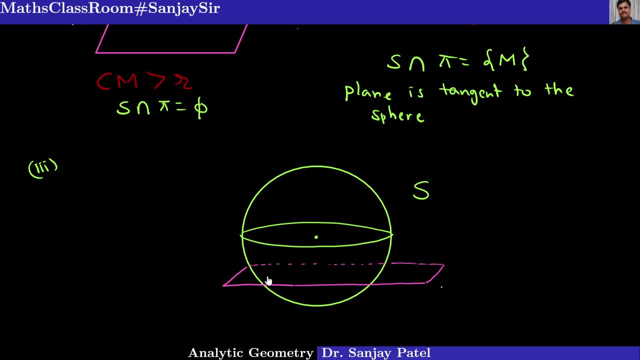 described here. so this is the intersection, this, the plane, is intersecting the sphere in infinitely many points in this case. so this is the center and we draw perpendicular of perpendicular from the center onto this plane. this is the foot of the perpendicular which i am calling m. 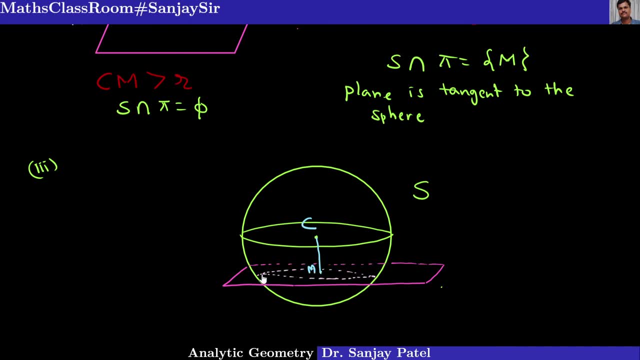 ok. so what i am getting here is again the intersection as a circle. so circle is our intersection set of the plane pi and the sphere s. so i can say, as intersection, pi is nothing but this circle. as shown in the figure, this m is actually the center of the. 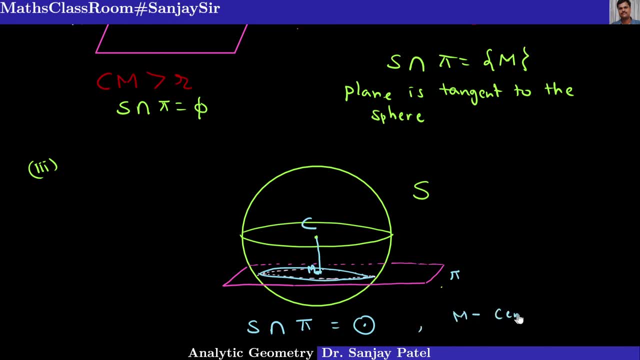 circle. just note down that m is the center of the circle of intersection. ok, and what is the radius of this circle of intersection, that you can immediately see that this distance, this distance is the radius of the circle of intersection? suppose this point is p, and if you